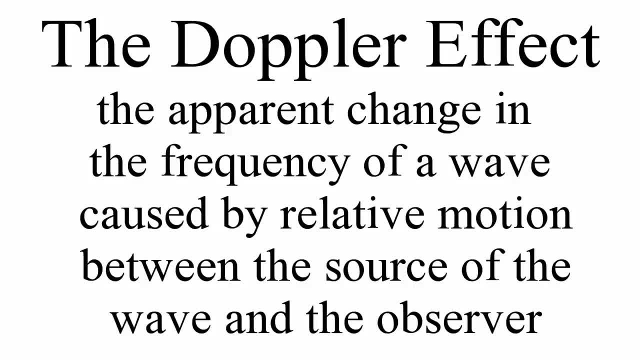 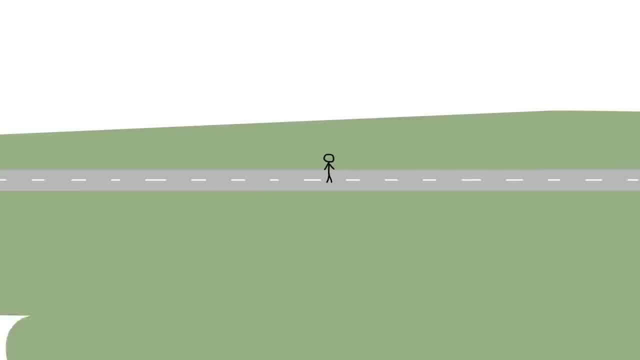 relative motion between the source of the wave and the observer. It makes sense, but it gets interesting when you can think of it as a motion of a blue disc. So what are the causes of the Doppler Effect to some of its applications? So let's say you are standing in the middle of a road. 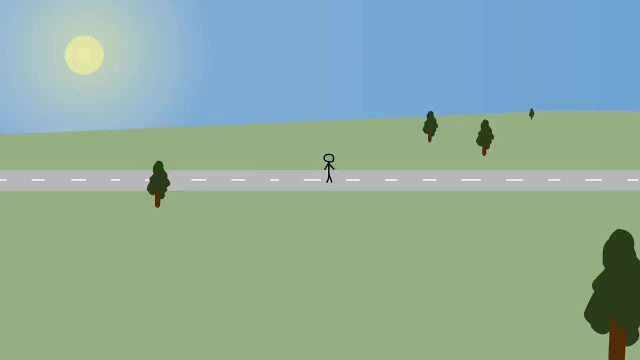 that's you and a car drives past you very fast As it does, so it honks its horn. because you're standing in the middle of the road, The horn to you might sound something like this: So it starts at a high pitch and moves to a lower pitch, even though from the driver's 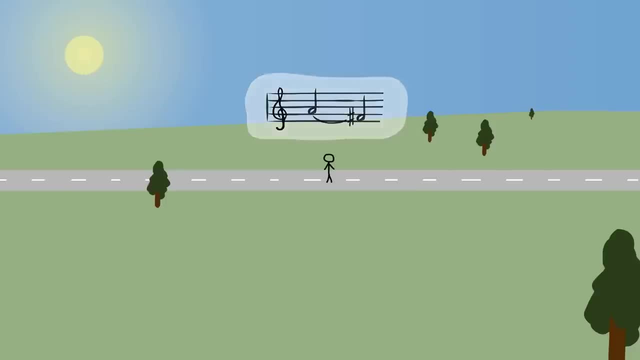 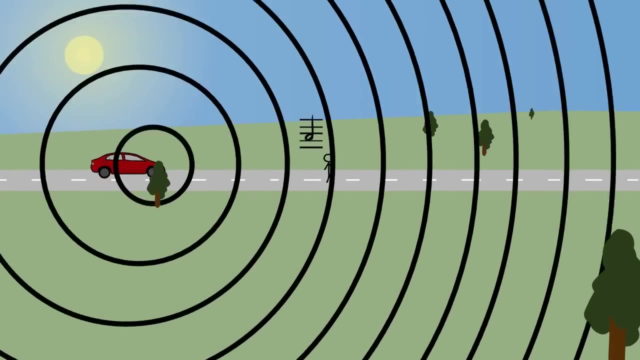 perspective, the horn is playing the same pitch the entire time. So what's going on? As the vehicle is coming towards you, the sound waves that it's emitting bunch up and so are delivered to you at a higher frequency, which you interpret as a higher pitch, because the 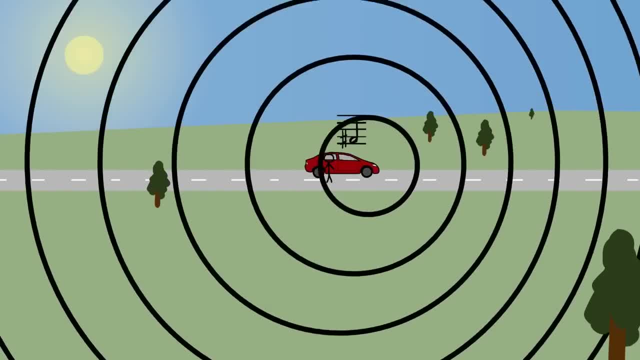 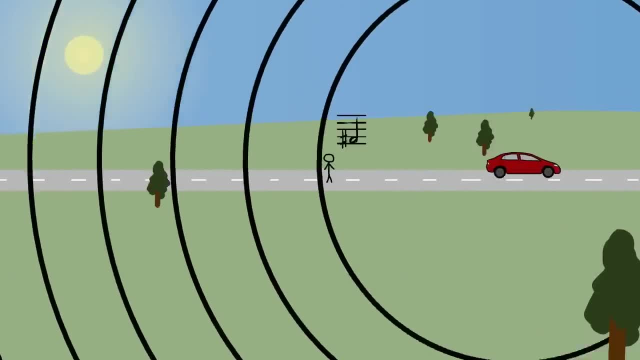 frequency of sound waves is pitch, And then, when the vehicle passes you and is moving away from you, the sound waves spread out and so you hear them at a lower frequency, a lower pitch. So that's how the Doppler effect works with sound. It also affects another kind of wave. light. So let's say you look at your observatory and you see that you have a low Pitch. So that's how the Doppler effect works with the sound It also affects another kind of wave light. So let's say you look at your. 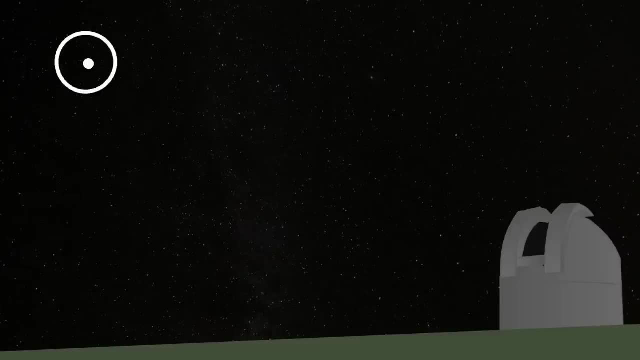 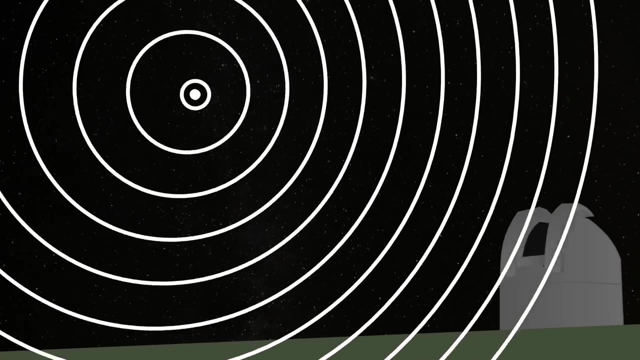 you see a star Just like the car's sound waves. if the star is moving towards you, even if it's a little bit, the light waves that it emits will be bunched up, meaning that you see the light at a higher frequency than it actually is. Frequency in sound is: 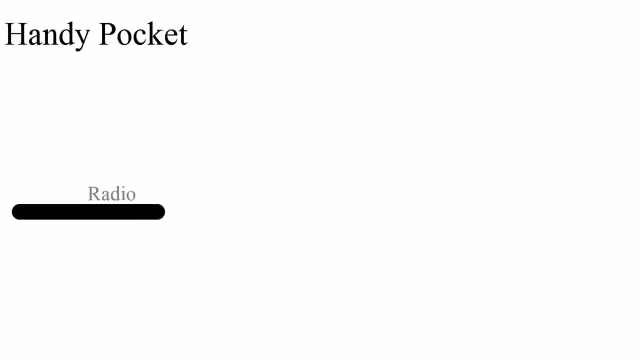 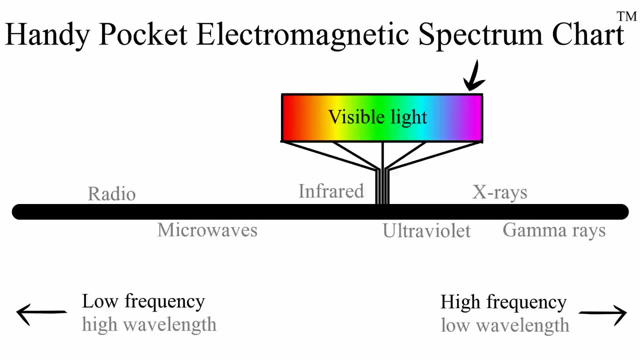 pitch. so what does it mean for light? Well, if we look at our handy pocket electromagnetic spectrum chart, we'll see that a small change in frequency for visible light will change its colour. Higher frequency light waves means bluer light and lower frequency light waves 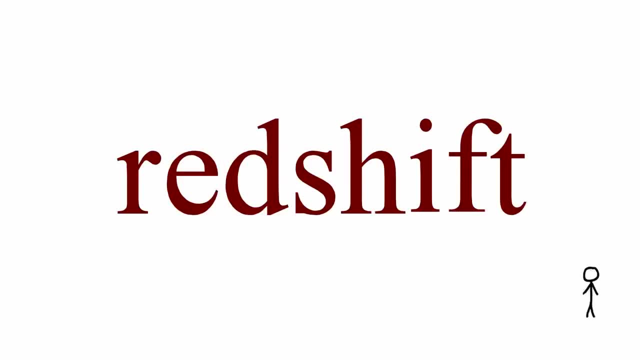 means redder light. This is called redshift and it may possibly be among the weirdest and coolest things of all time. Stars, or anything that you can see, change colour depending on their relative motion to you. Of course, you can't see this minute difference with. 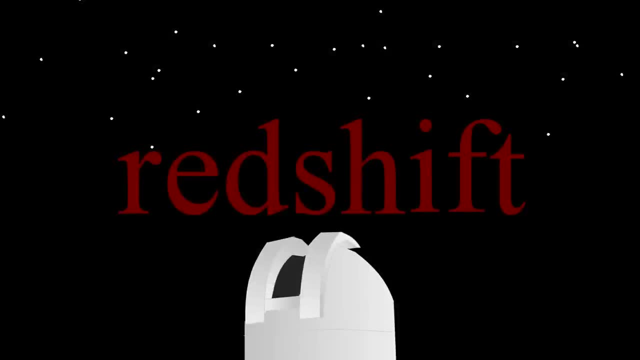 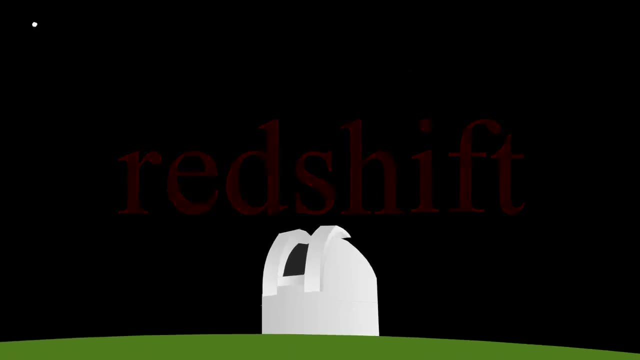 your eyes, but astronomers with the right equipment can use this effect to tell whether stars are moving away from or towards Earth. As it turns out, almost everything we can see in the universe is moving away from us very quickly, which is both an important piece of evidence for the Big Bang and an